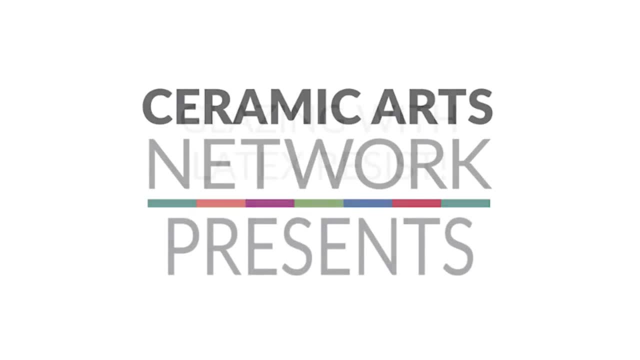 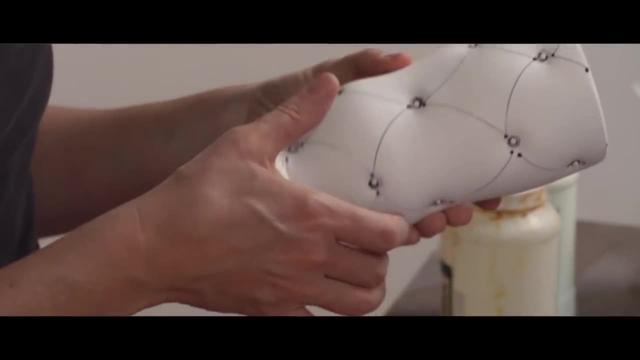 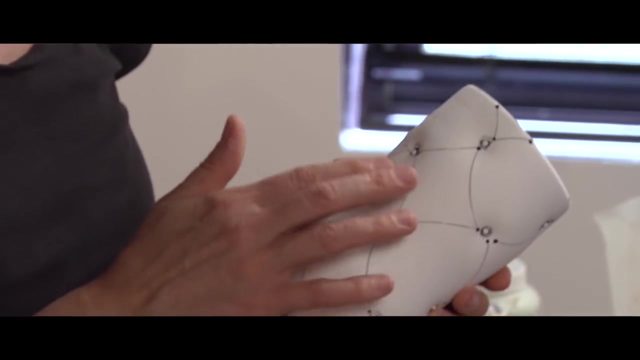 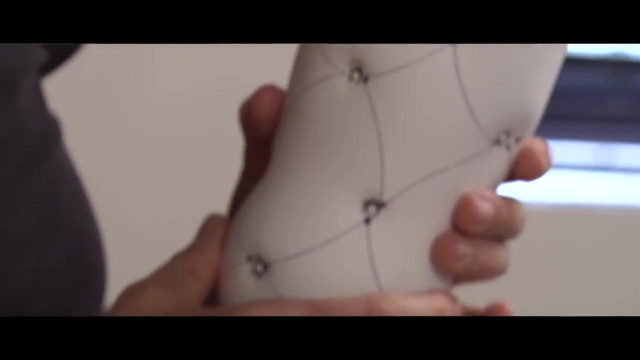 I'm going to do two different layers of glazing on here and the nice thing about the jet black- Amaco jet black under glaze is that it'll show through glaze and slip, so it really will show through multiple layers if, with the exception of opaque or matte glazes, sometimes it won't show. 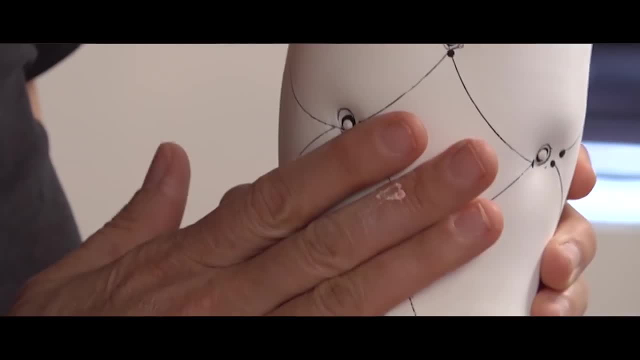 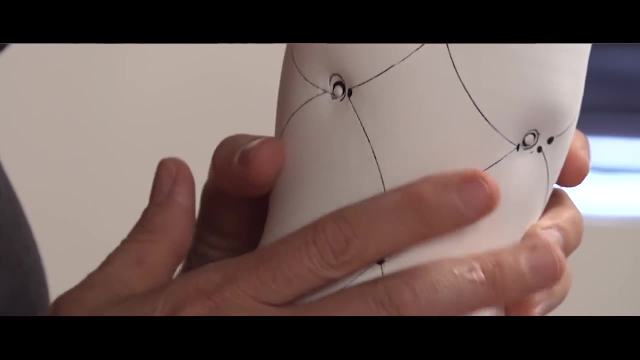 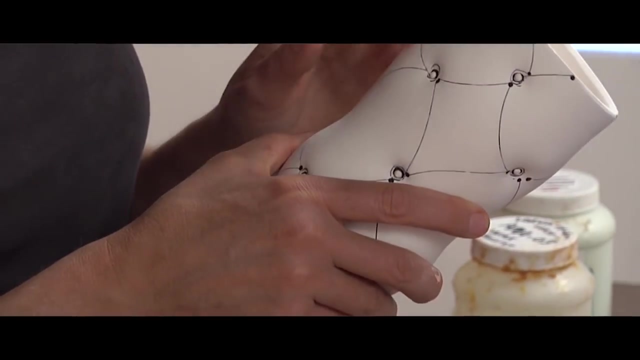 through. but what I use for this pattern is flashing slip, which basically is a slip with a clay that will change color according to atmospheric firing and then a celadon glaze over it. so the black slip decoration will show through both of those layers. so I'm going to 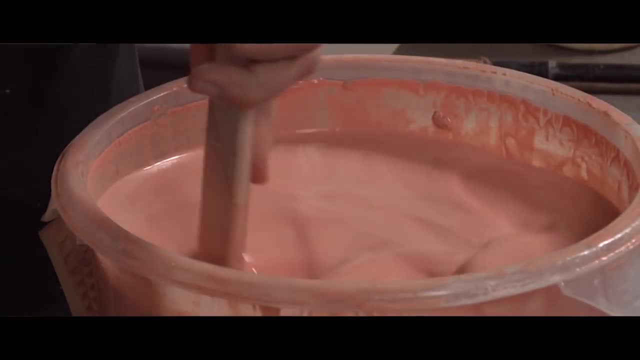 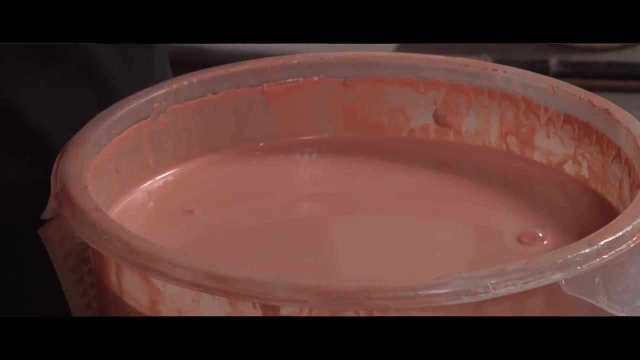 start with dipping it in a flashing slip which is called bisque flash and it's formulated for bisque ware. so I'm going to dip this in my already bisque cup. so I've waxed the bottom foot ring so the glaze stays off there, and then I'm just going to do a quick dip in the flashing. 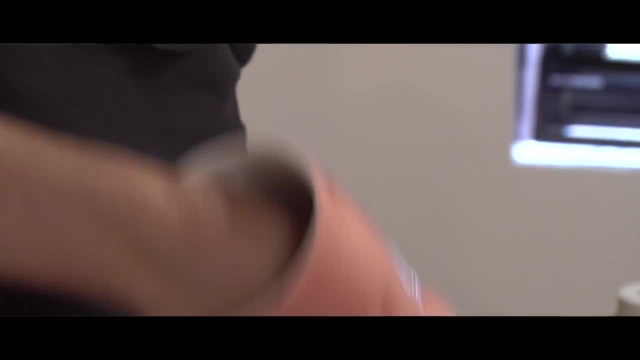 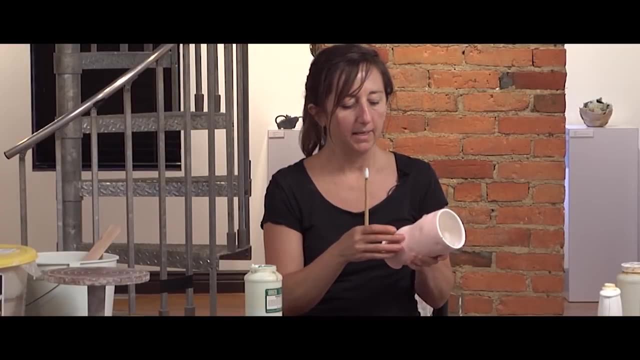 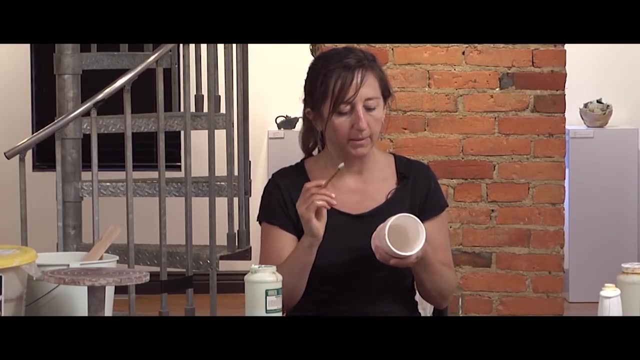 slip up to the rim and then set it aside to dry before I use the latex resist. I've dipped this in the flashing slip and it's dried and you can see where the slip inlay lines are, because it raises up a little bit through the flashing slip. so then I'm going to go back with my rubber. 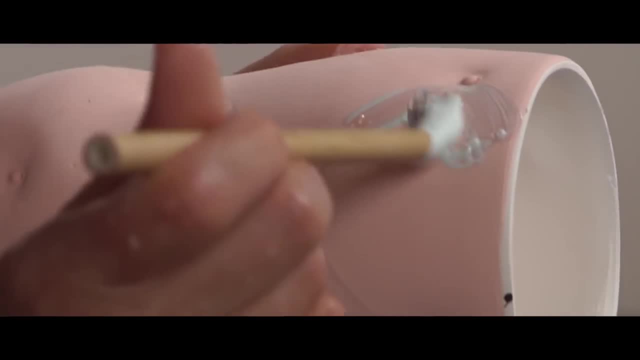 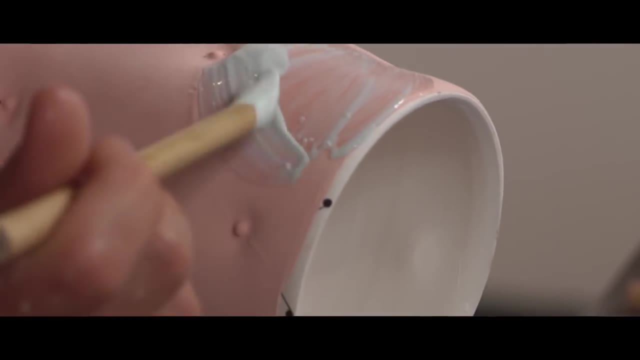 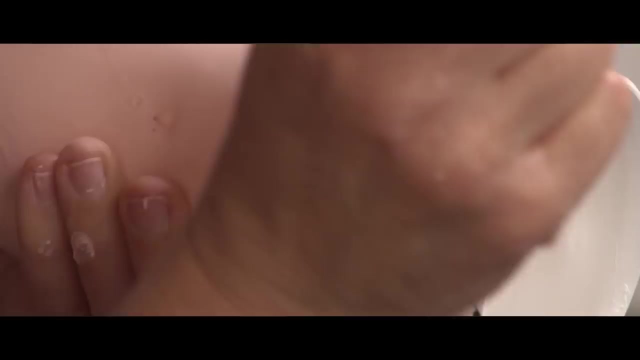 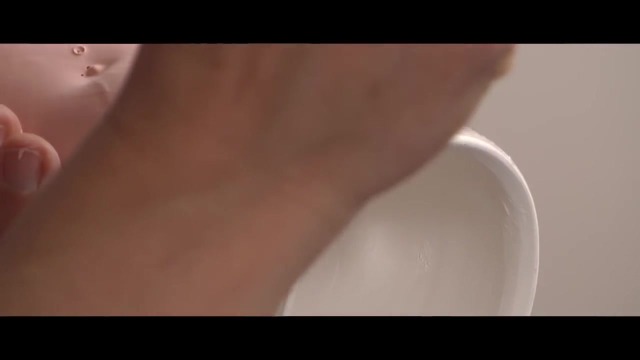 latex and I'm gonna paint everything that's not a diamond in the pattern. so you'll see the pattern start to take effect here in a second. So this is going to show how you can paint latex over a slip glaze, dip it in another color and then peel it off again. 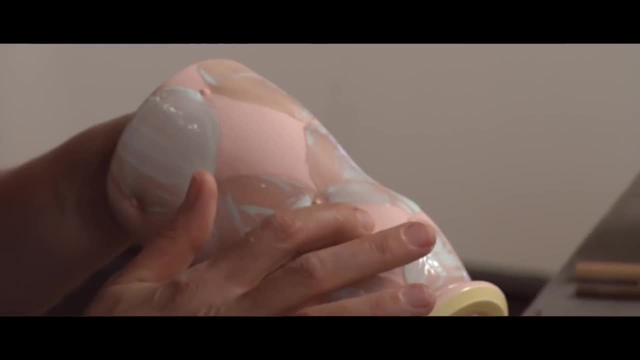 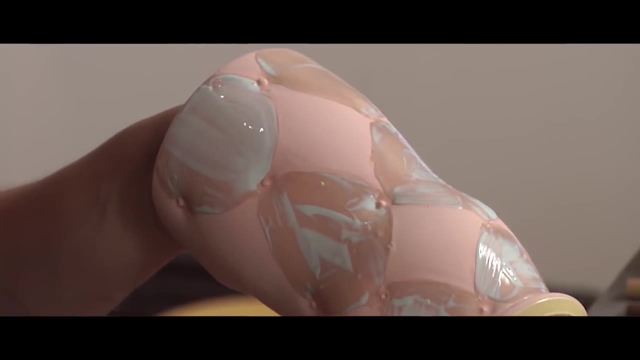 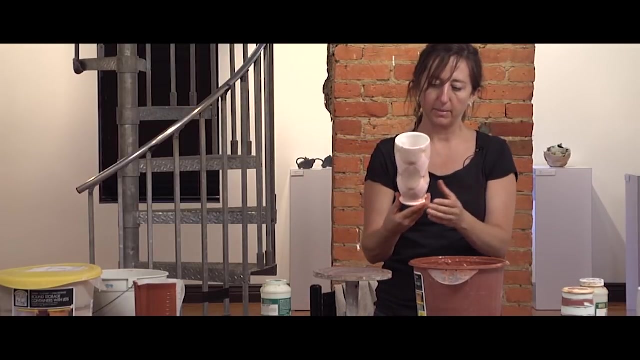 So now you can see that the diamond pattern is what's left, and so when I dip it in the Celadon, these will be glazed and then the rest will be peeled off to reveal the flashing slip underneath. So I painted the latex over my flashing slip and given it time to dry, and now I'm going.